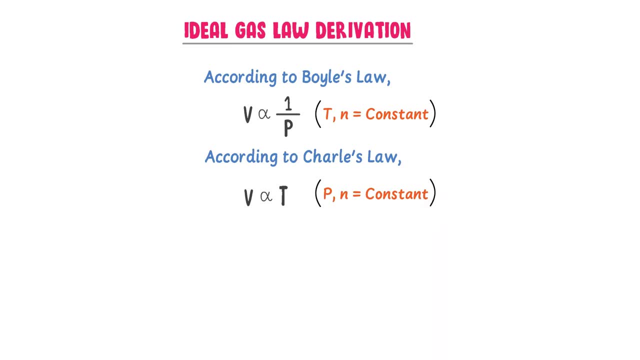 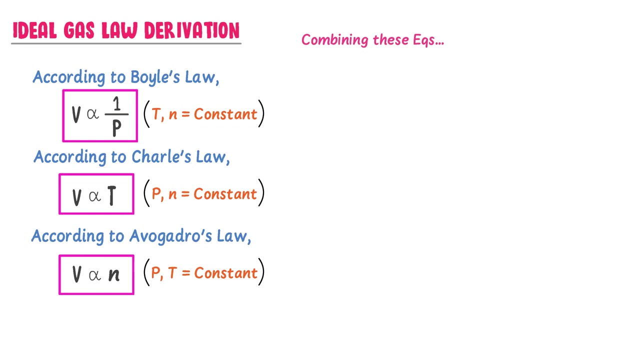 while keeping pressure and number of moles and constant. Thirdly, according to Avogadro's law, volume is directly proportional to number of moles and while keeping pressure and temperature constant. Now I combine all these three equations I get volume is inversely proportional. 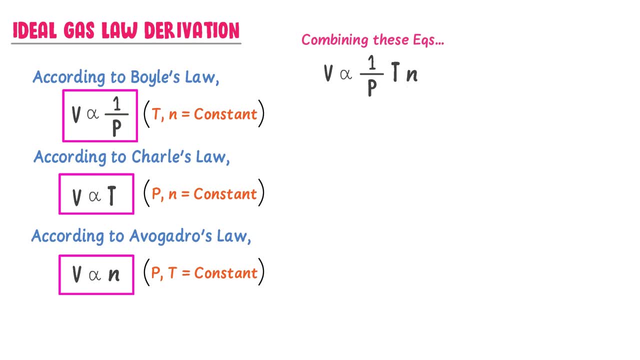 to the pressure directly proportional to temperature and number of moles. Here, to eliminate the sign of proportionality, we need to put some sort of constant. I get v is equal to r and to 1 upon p and to t and to n. Remember that. 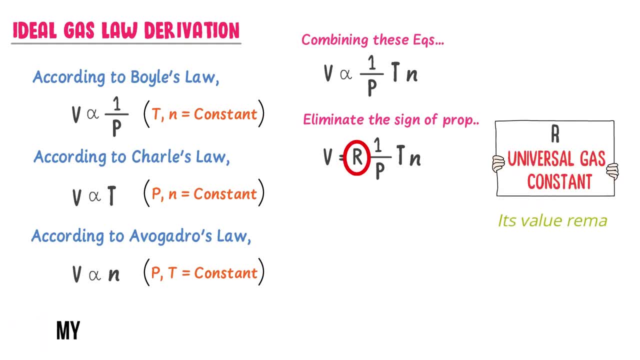 r is the universal gas constant. Its value remains the same for all gases. That's why it is called as universal gas constant. Now I shift p from the right-hand side to the left-hand side, I get pv is equal to nRT. This is the ideal gas law or general gas equation. 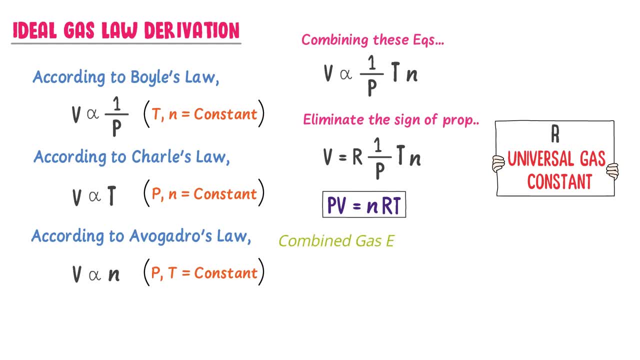 Some people also call it combined gas equation, because all these laws of gas are combined together to form this equation. Now I shift n and t from the right-hand side to the left-hand side, I get pv upon. nT is equal to r. Here r is constant. 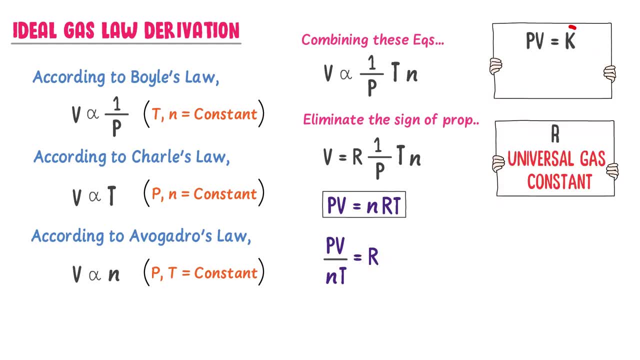 We know about Boyle's law: pv is equal to k. k is constant, so we write: p1v1 is equal to P2V2.. Similarly, R is constant, So we write: P1V1 upon N1T1 is equal to P2V2 upon N2T2.. 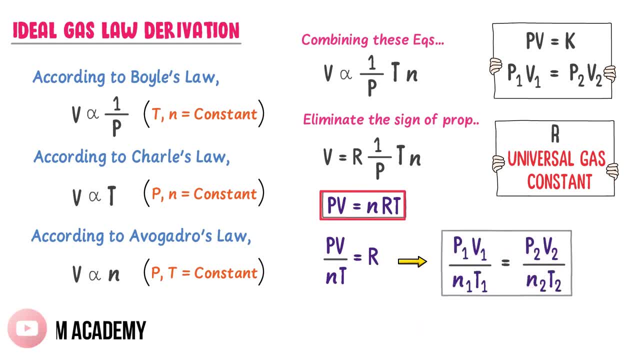 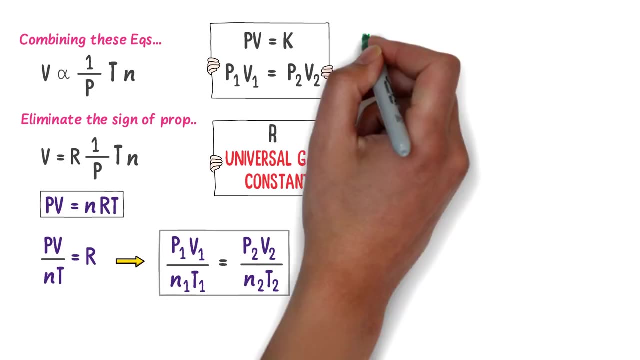 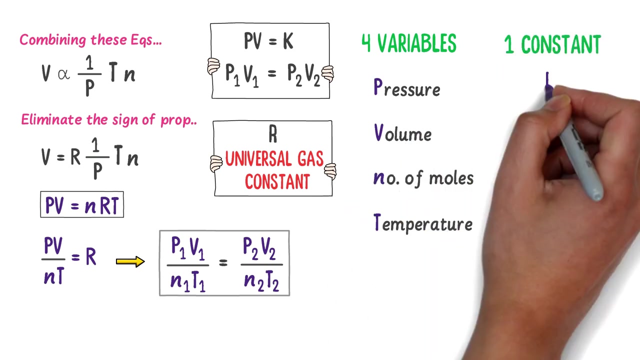 Remember that we will often use this equation: PV is equal to NRT and this equation: P1V1 upon N1T1 is equal to upon N2T2.. Just note it down: these both equations. Now, remember that there are four variables: pressure, volume, number of moles and temperature, While there is one gas constant. 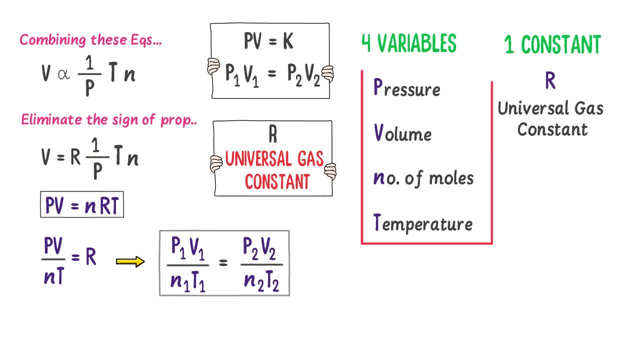 universal gas constant R. So, out of these four variables, the value of three variables would be given and we have to find the value of one variable. For example, the value of volume would be given and the value of volume would be given. So, out of these four variables, the value of 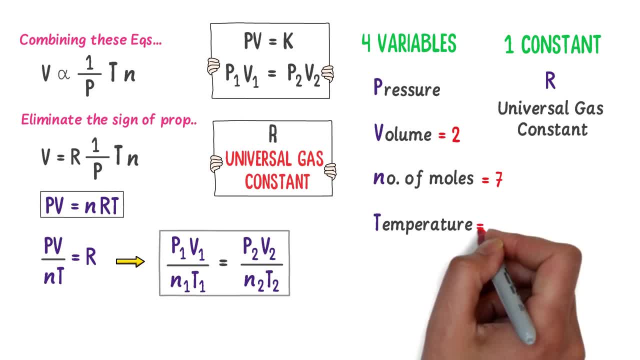 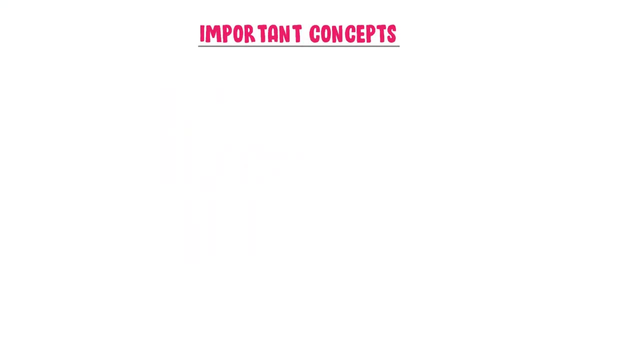 number of moles would be given and the value of temperature would be given, and we would be asked to find the value of pressure. Thus, we will find the value of pressure using ideal gas equation. Now let me teach you some important concepts of ideal gas equation, For example. 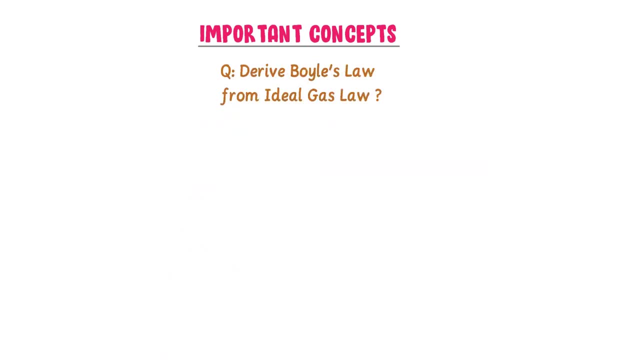 derive Boyle's law from ideal gas law. Well, let me write: P1V1 upon N1T1 is equal to P2V2 upon N2T2.. We know that we derive Boyle's law at constant temperature and keeping the number of. 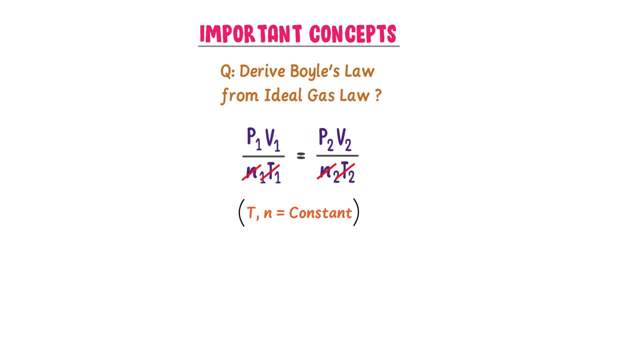 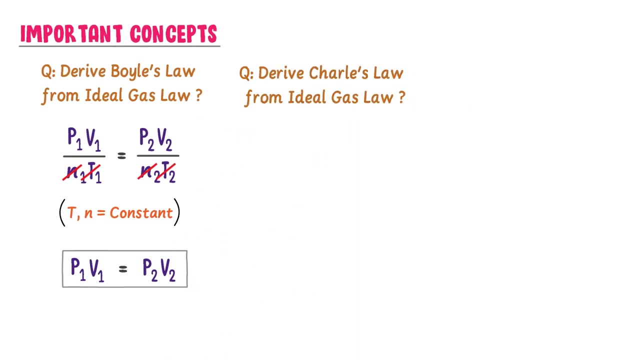 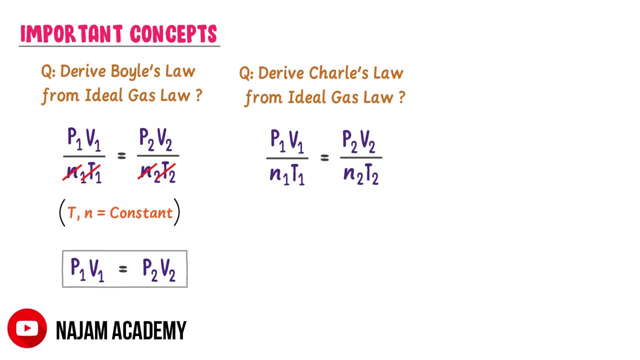 is equal to P2, V2 upon N2, T2.. We know that we derive charge law at constant pressure and number of moles remain the same, So I cancel the constant variables in this equation. I get: V1 upon T1 is equal to V2 upon T2.. This is the charge law and the required proof. 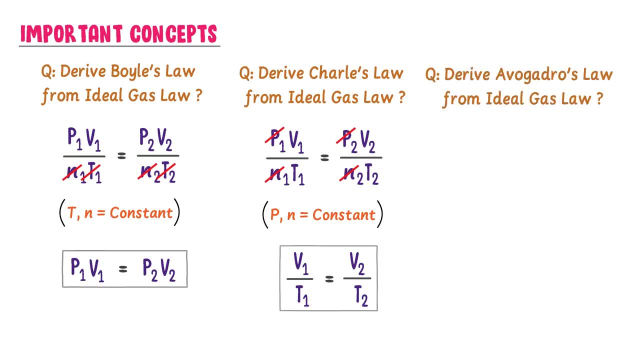 Similarly derive Avogadro's law from ideal gas law. Well, let me write: P1 V1 upon N1 T1 is equal to P2 V2 upon N2 T2.. We know that we derive Avogadro's law at constant temperature. 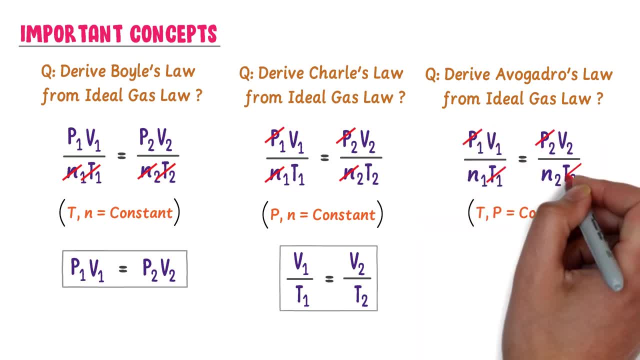 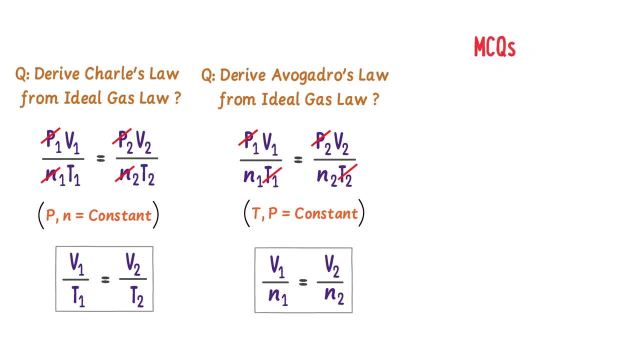 and pressure. Thus I cancel the constant variables in this equation. I get: V1 upon N1 is equal to V2 upon N2.. This is the Avogadro's law Here. let me teach you my personal MCQs. At standard pressure, the ideal gas equation. 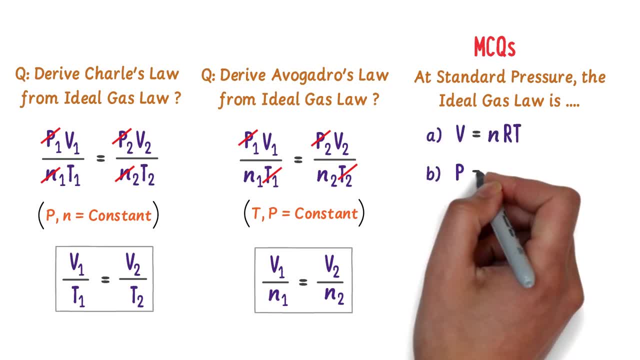 is: V is equal to NRT, P is equal to RT, V is equal to RT And PV is equal to RT. Can you guess the correct option? Well, we know that standard pressure, P is equal to 1 atmosphere and at standard pressure, number of moles N is equal to 1 mol, The ideal gas. 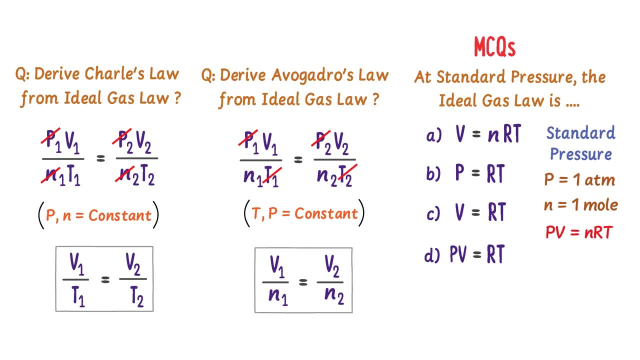 equation is: PV is equal to nRT. thus, putting the value of pressure and n in this equation, We get V is equal to RT. Thus the correct option is C: V is equal to RT. Therefore, noted down all these important concepts of ideal gas law. Now let me derive the value of universal. 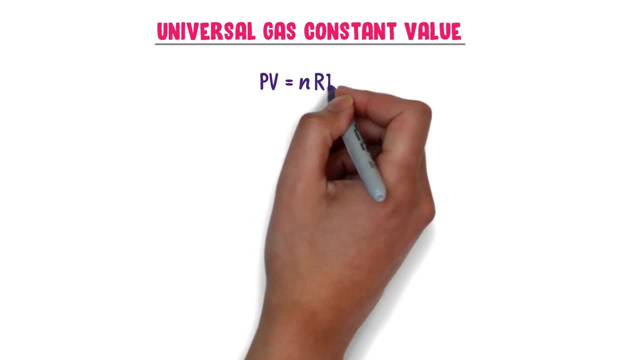 gas constant. We know that PV is equal to nRT. Shifting n and T from the right hand side to the left hand side, we get R is equal to PV upon nT. Now consider ideal gas in this closed cylinder at STP. STP means standard temperature and pressure. Remember that at. 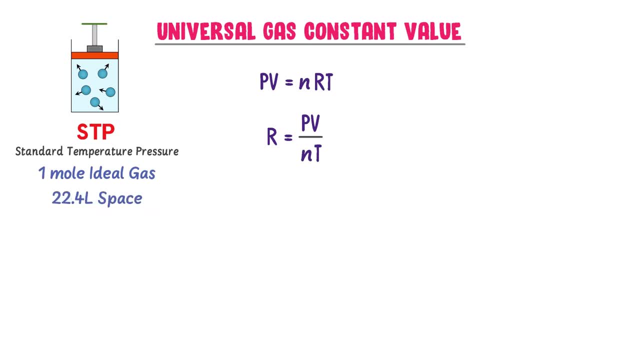 STP, one mole ideal gas occupies 22.4 liters space. So standard temperature is 200 degrees 273 kelvin, Standard pressure is 1 atmosphere, The volume at STP is 22.4 liter and the number of moles is 1.. Thus I put all these values in this equation I get: R is equal to 0.02. 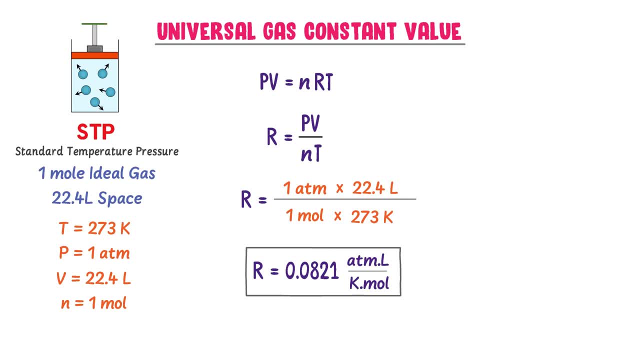 at 1 atmosphere liter upon kelvin mole. This is one value of the universal gas constant. Some other values of universal gas constants are At point: 314 joule per kelvin mole: 1.9. at 7 kel per kelvin mole: 0.0. at 3 bar dm cube per kelvin. 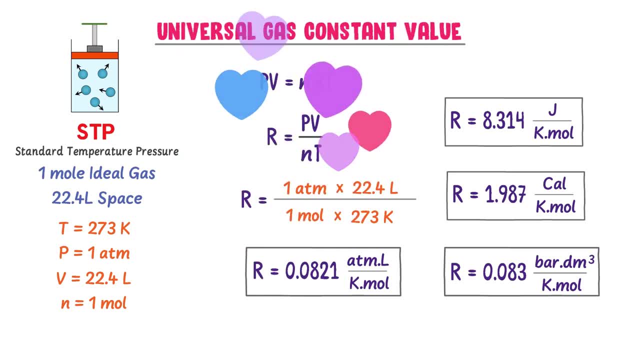 mole, etc. So these are the different values of universal gas constant. In the next lecture we will learn all about the values of universal gas constant and its link will be given in the description.